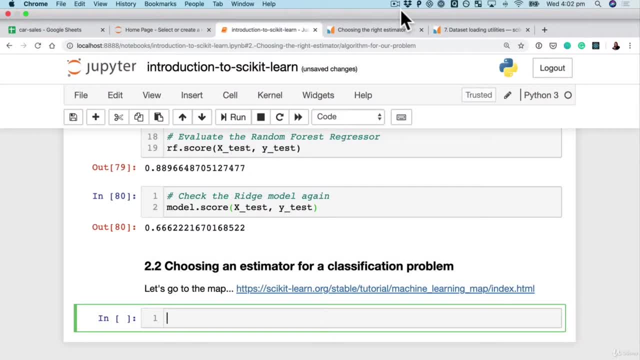 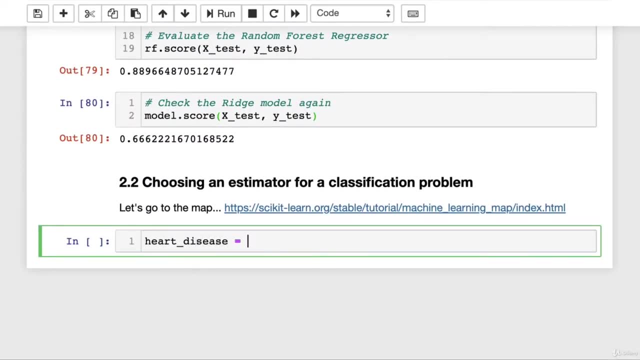 Alrighty. so we've seen how to choose an estimator for a regression problem. How can we do the same for a classification problem? Well, first of all, let's get a data set that is a classification problem back in our MITS. So we want data. We've already imported this above, but we're just going. 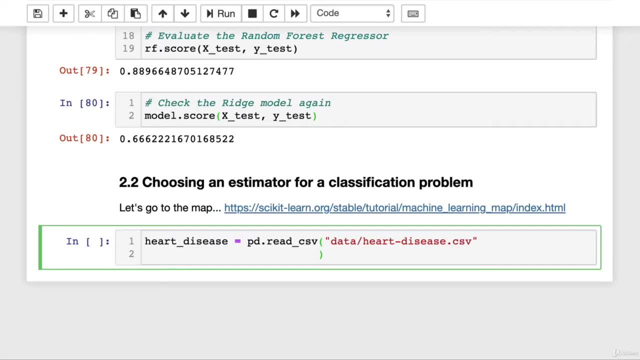 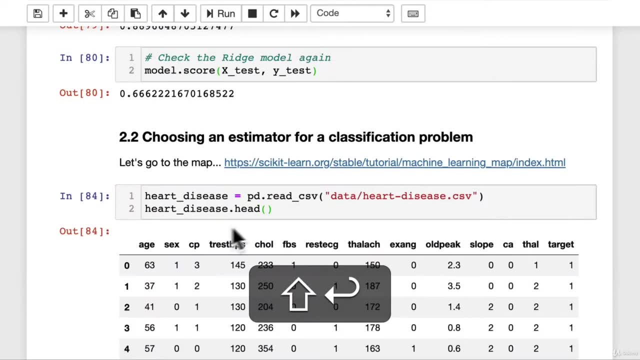 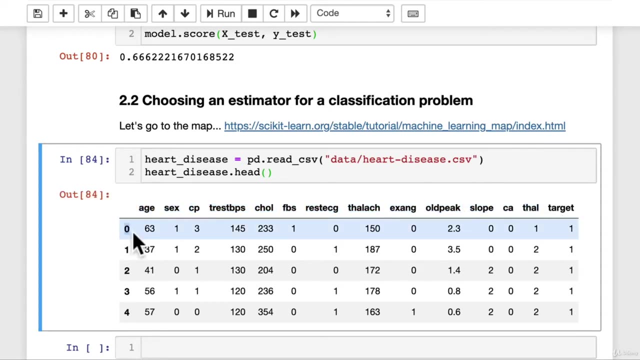 to do it again, just so we have it CSV, just to make sure it's the same: Heart disease, heart disease, dot head, Wonderful. So again we've seen this data set before. We want to use these columns of patient. Each row is a patient, so each sample is a patient, Each column or each. 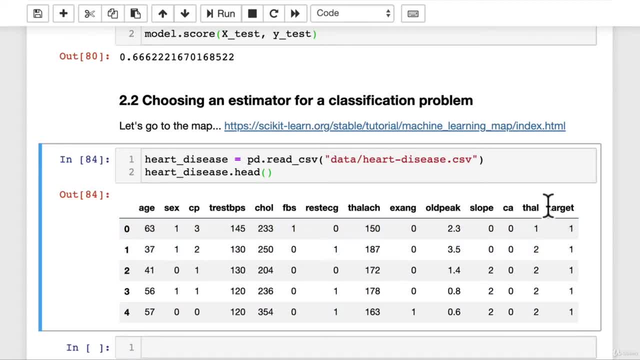 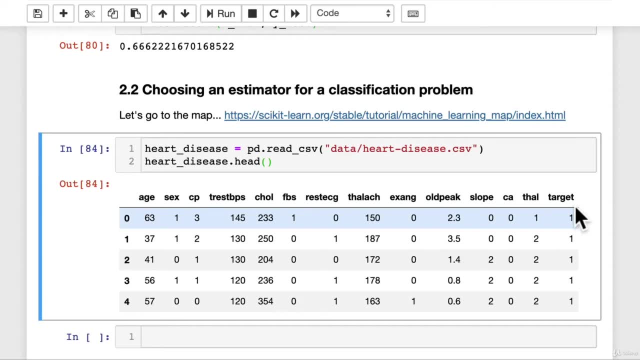 feature is a health attribute of that particular patient and the target, one or zero, is whether that patient has heart disease or not. So our model classification predicting something is one thing or another- heart disease or not. that's what we need. So what we're going to, 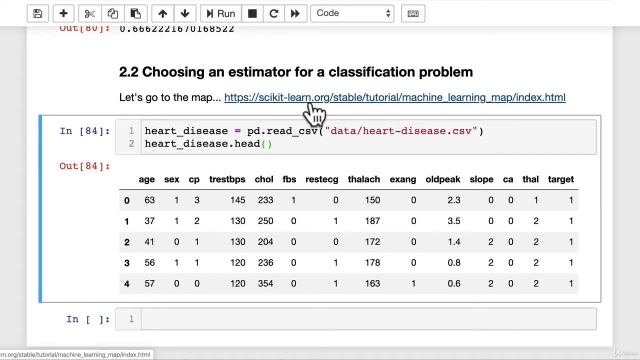 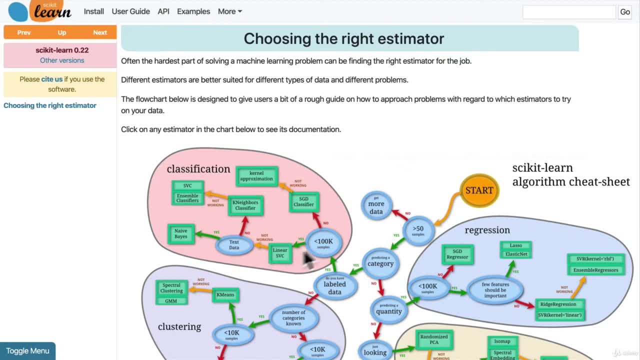 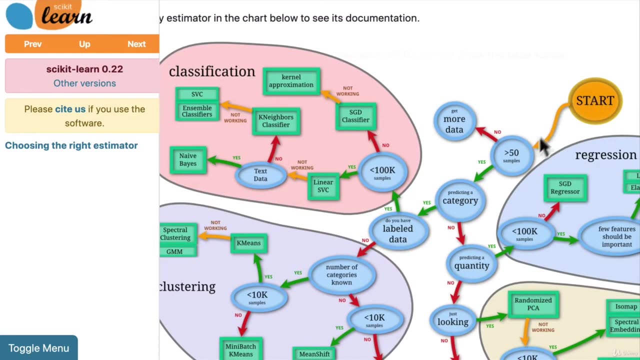 do is we left ourselves this little link here to go visit the map. So we're going to pay attention to that. We go here So we know we want something in the classification realm, but what we're going to do is we're going to start from the top and follow this through. So start Do we have above. 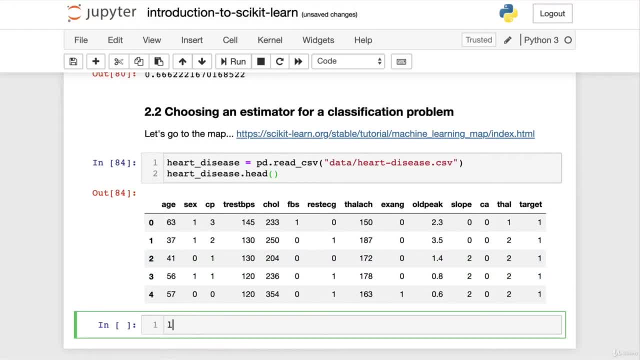 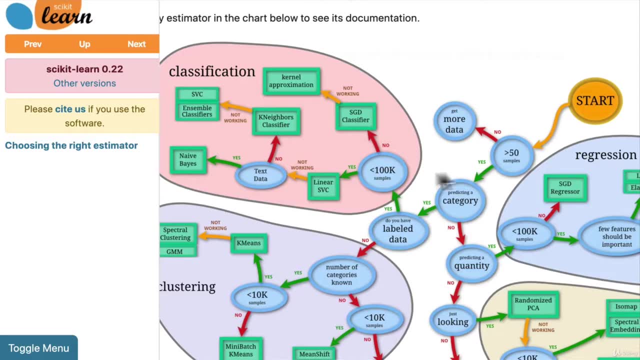 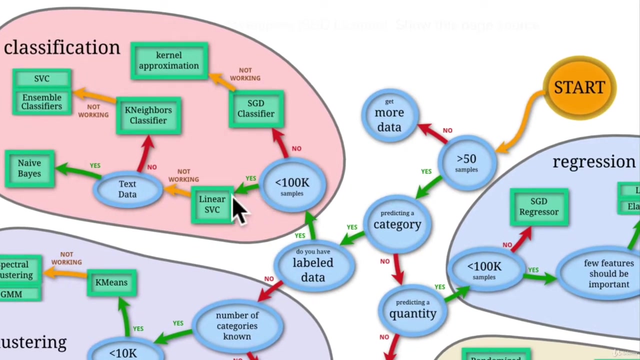 50 samples. Well, let's check. Each row is a sample. So we want Len heart disease 303.. Yes, we can. Are we predicting a category? Are we Heart disease or not? heart disease Sounds like a category to me, Yes. Do we have labeled data? Yes. Do we have under 100k samples? Yes, What is this? 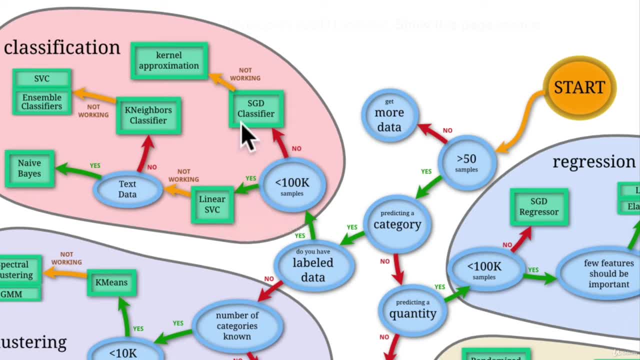 We reach a little green box, Beautiful. So remember, the green boxes are estimators or machine learning algorithms. So let's have a look. This is telling us our problems: classification, and maybe the first one we come to is trying a linear SVC. 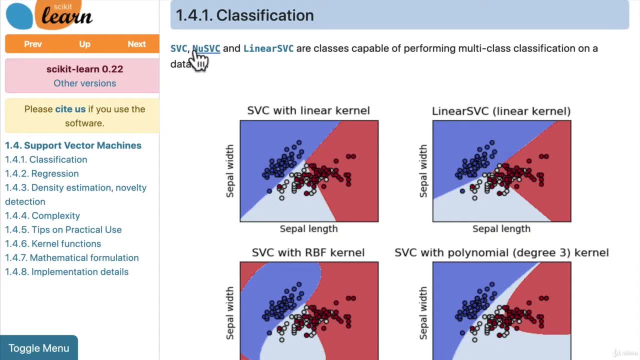 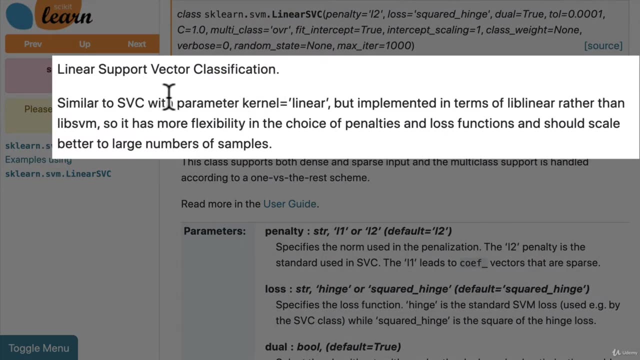 Well, all right. Classification: SVC and linear SVC are classes capable of performing multi-class classification on a dataset. Well, this one particularly said linear SVC, So let's have a look. Linear support vector classification: Similar to SVC with parameter kernel: linear. 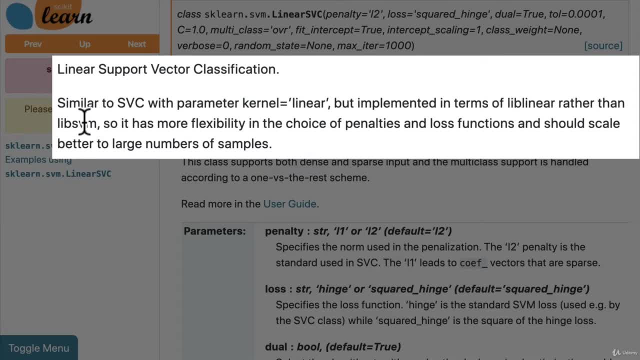 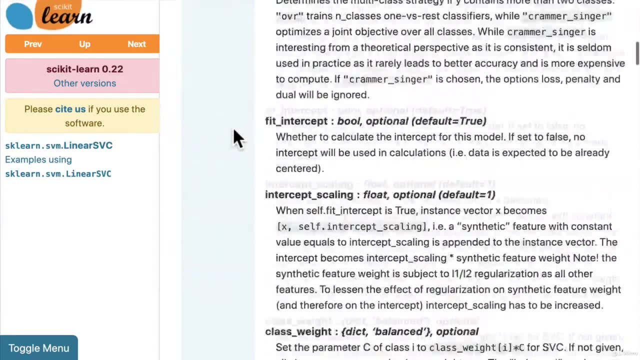 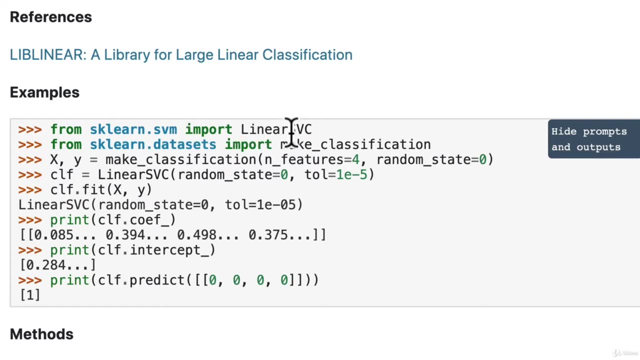 but implemented in terms of lib linear rather than lib SVM. That's a lot of terms there And most of them I don't really understand. But what's important here is that if we go down to the code example, we can see from sklearnsvm import linear, SVC, X, Y- Oh, they've used X and Y. 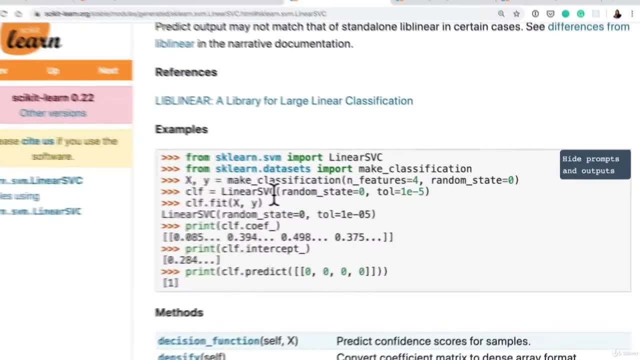 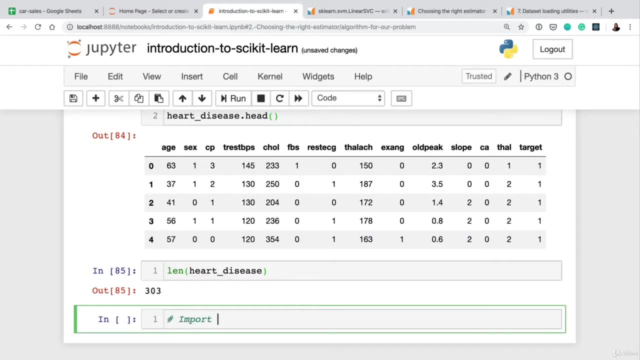 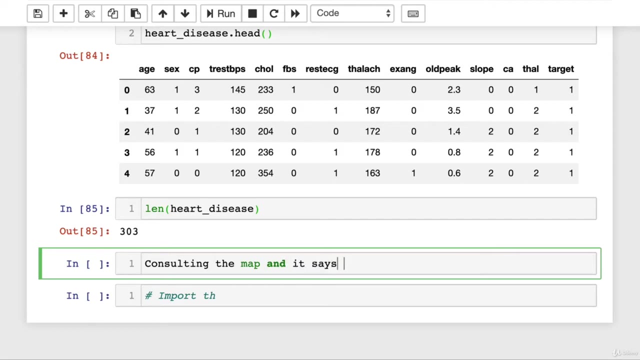 CLF classifier equals linear SVC. All right, This is kind of similar. Well, let's not take the documentation's word for it, Let's try it for ourselves. We'll go import- Actually, we'll leave ourselves a note- Consulting the map, And it says to try. 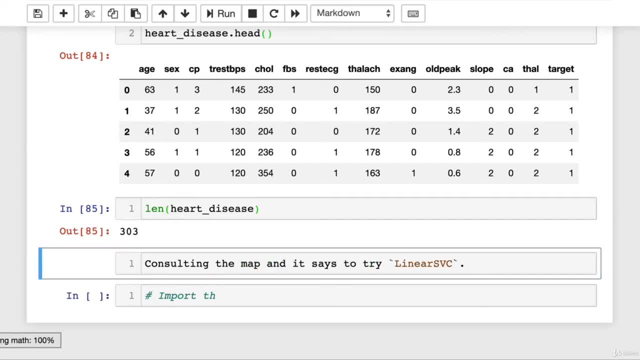 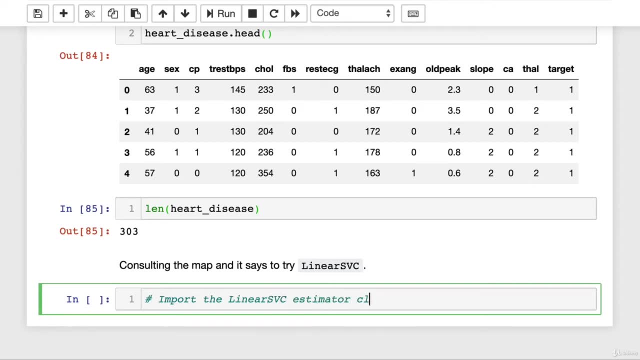 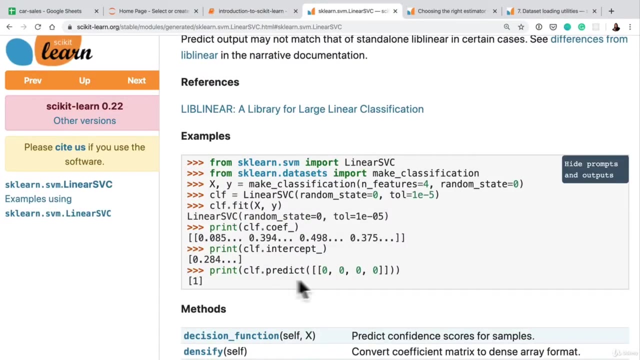 out linear SVC. So that'll be our first port of call: Import the linear SVC estimator class. I'm going to go from sklearnsvm And really what I'm doing here is I'm basically just going to rewrite this, but for our problem. So sklearnsvm: import linear SVC. 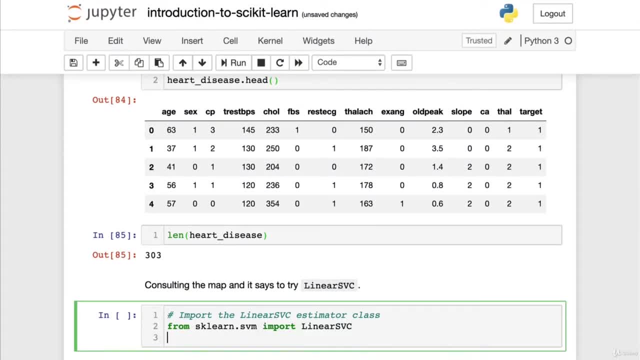 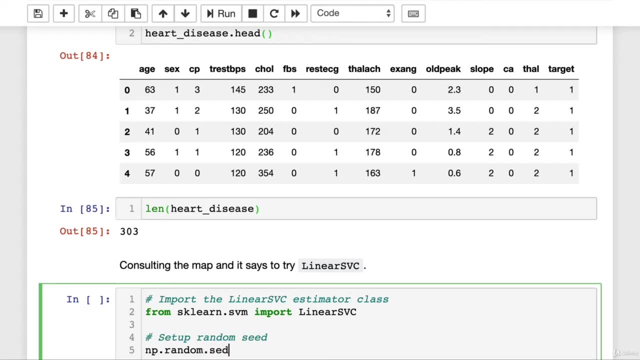 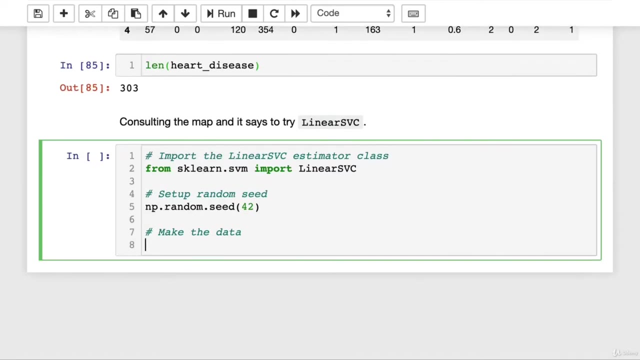 Import linear SVC. Wonderful, Set up random seed, Mprandomseed, And we'll use our fateful42.. And then we're going to go make the data. We saw this in the previous section. Section one: Get your data ready. 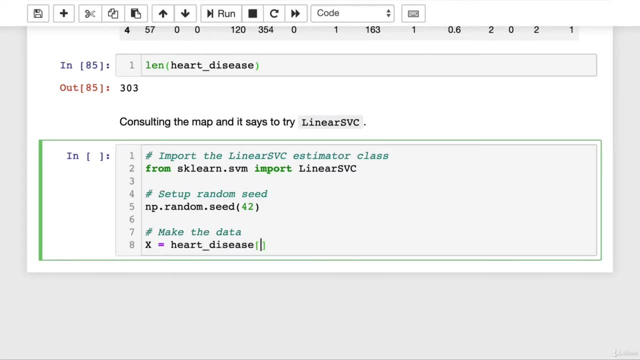 X equals heart disease, dot drop, And we want to get rid of the target column on axis equals one And Y equals heart disease. Y is actually the target column, beautiful, and then we're gonna go split the data. next test: oh no, train comes first, silly me. I've done this about a hundred times by now and still. 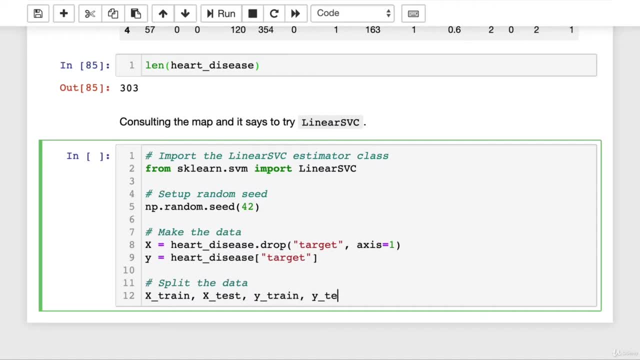 getting it wrong. see, this is what it takes. it takes a little bit of practice or it takes a lot of practice to start applying, start becoming machine learning practitioner, knowing how to deal with data, knowing how to split data, knowing how to model data. it's all part of the practice. test size. yes, that is correct. 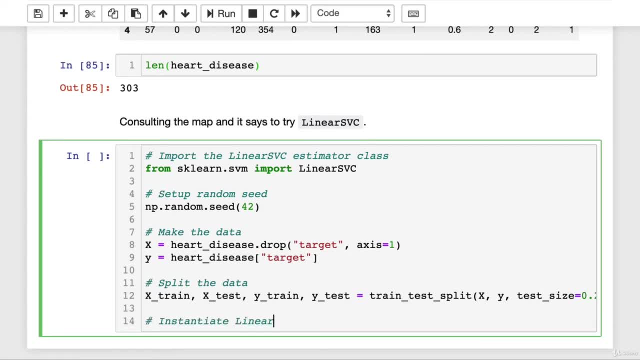 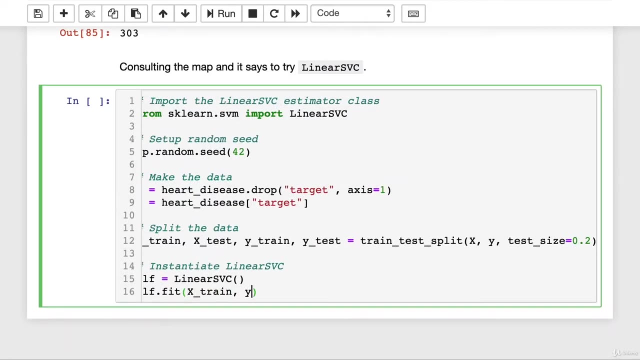 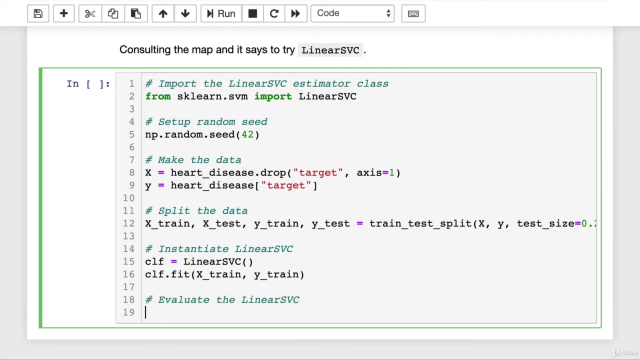 that's what we want to do: instantiate linear SVC. so we'll call it CLF, short for classifier, linear SVC, and we're gonna go that'll do actually CLF dot fit. we want X train, Y train, and then we're gonna go evaluate linear SVC, CLF dot. 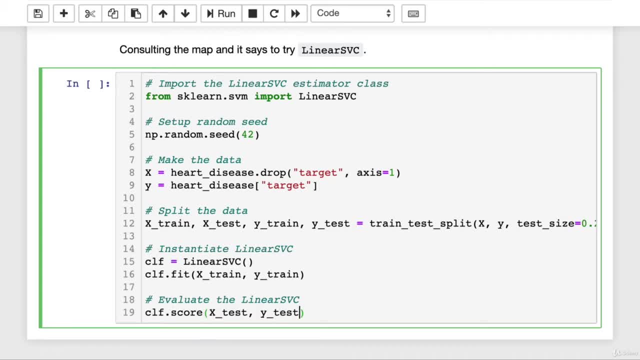 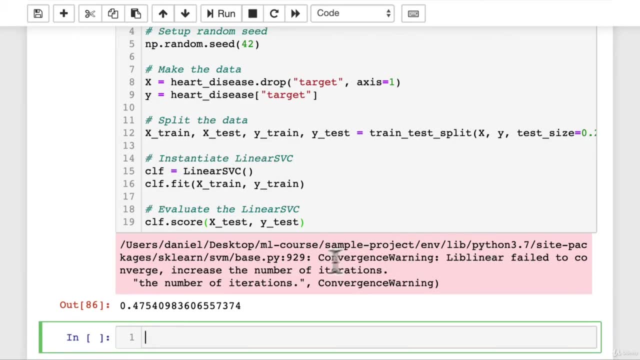 score: X test, Y test: all right, beautiful, let's say this in action. wonderful: live linear. fail to converge, increase the number of iterations. well, this is one of those things where, if you came into an error like this, what I might do is go convergence warning or Google this message and see what came up. 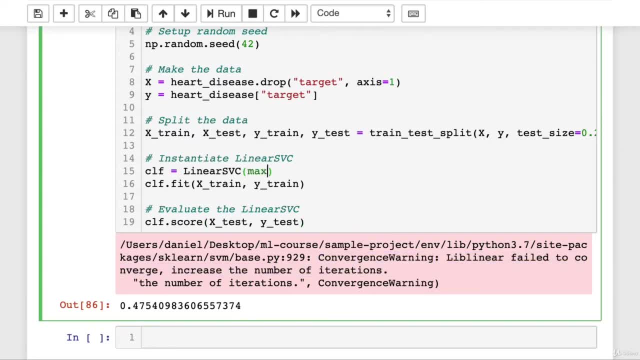 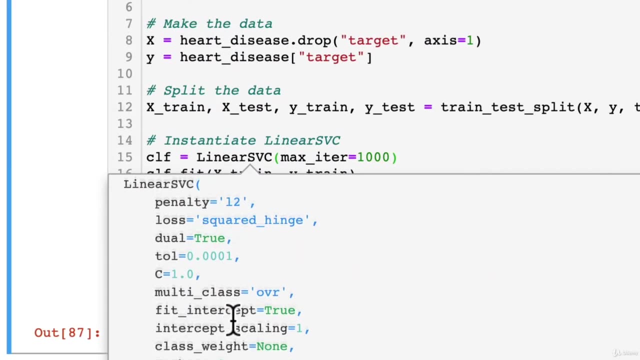 because I've had a little bit of experience with it. I might do something like: max it equals a thousand and it still happens, right? so increase the number of iterations. we've done that, we've gone. max iter equals 1000, but this is actually how much does it start Max iteration? oh, it's default. 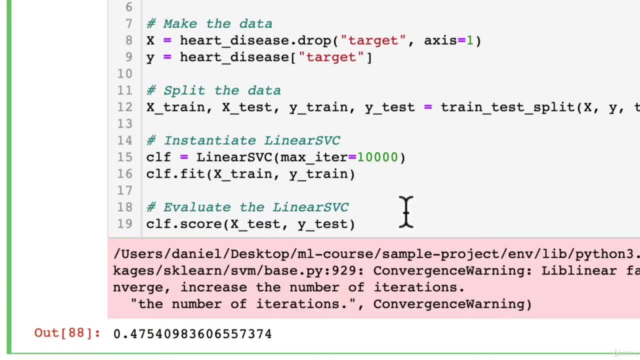 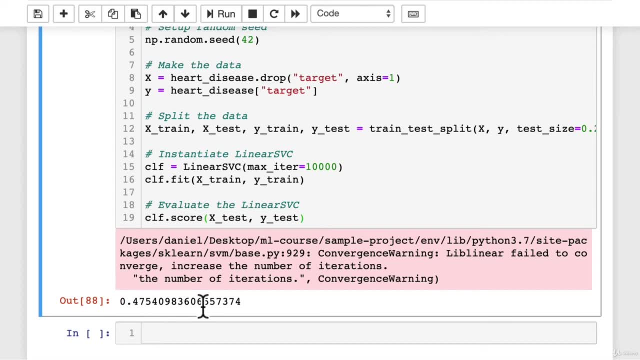 by 1000,. let's see 10,000, still there. Well, let's bypass that for the time being. we're getting a warning and see here, the score is below 0.5,. now, why is that a trigger? 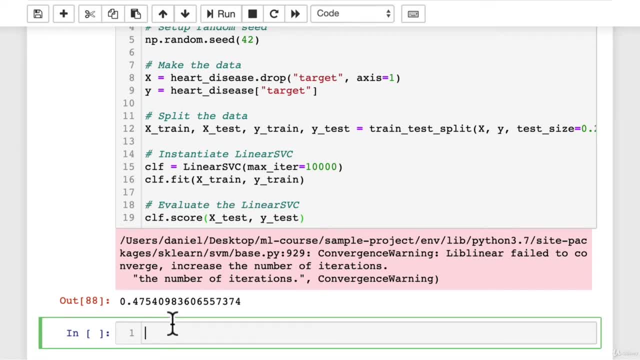 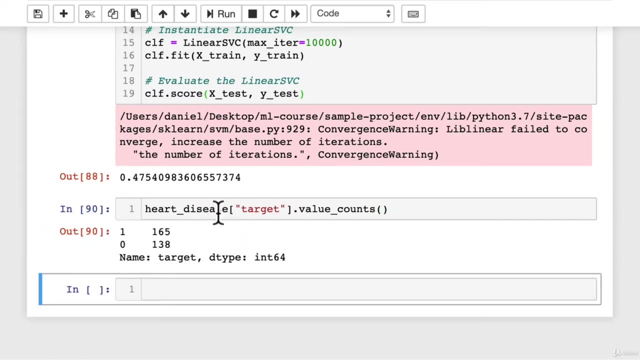 in our heads. Well, because if we look at our data, we want heart disease target dot value counts. so we see there's only two classes, one or zero. does someone have heart disease or not? Right, so it's a binary classification problem. binary meaning. 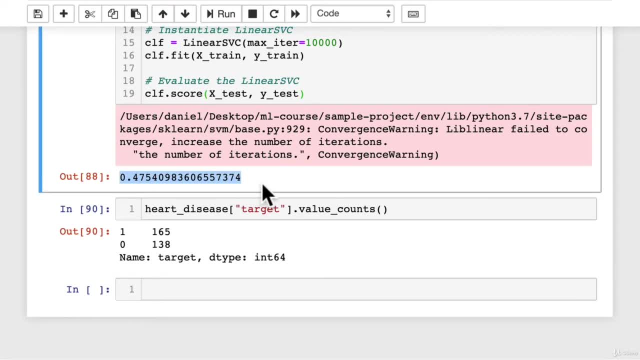 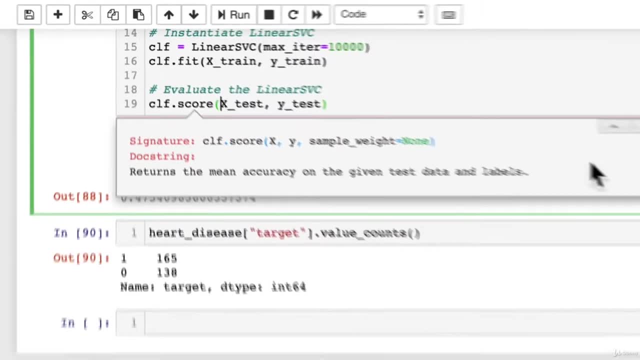 one or the other and our model is receiving a score of 0.47, returns the mean accuracy on a given test data and labels. as I said, we'll look into evaluation metrics in a future section, but what you can imagine this is our model is only. 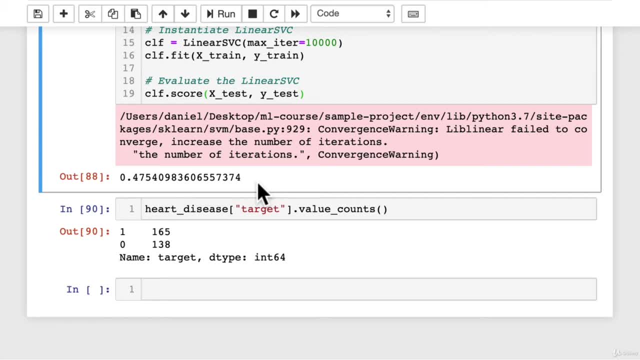 operating at 47% accuracy. and why does that trigger us? Well, because there's only two classes. so that means, if we were just guessing whether someone had heart disease or not, based off their health attributes, we were just guessing yes or no. 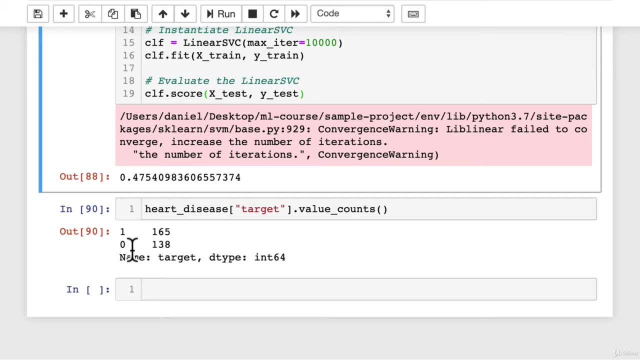 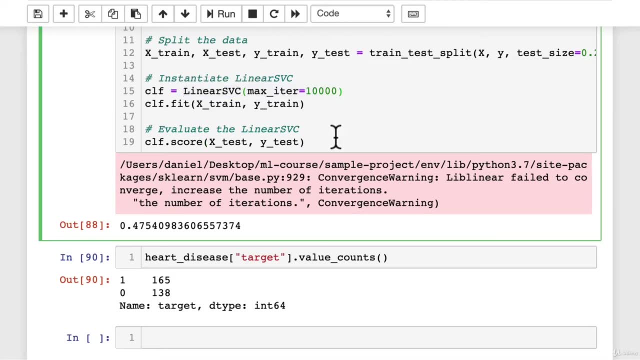 we would get 50%. it's basically a coin toss. so what's that triggering in our head? It's saying, hey, without fixing this warning or without improving our model by tuning the hyperparameters, our linear SVC model might not be. 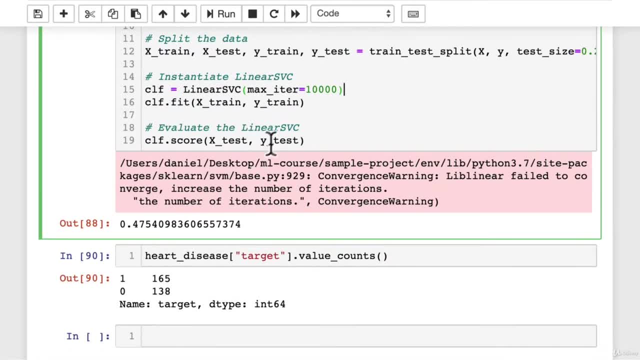 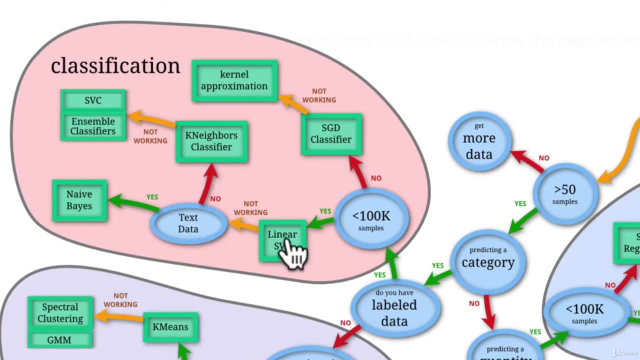 finding patterns between X and Y. so what can we do? Well, when in doubt, come back to the graphic: not working. are we working with test data? Because we just tried linear SVC, so we're going to say not working. are we working with test data? No, 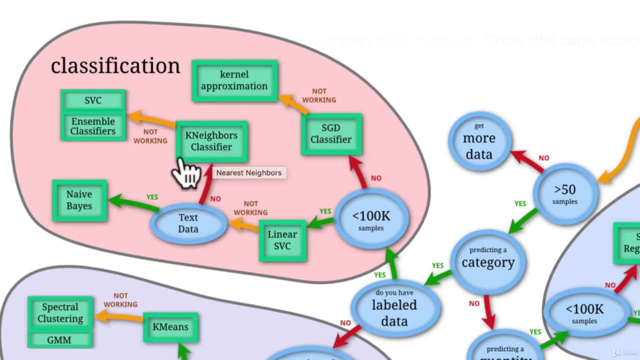 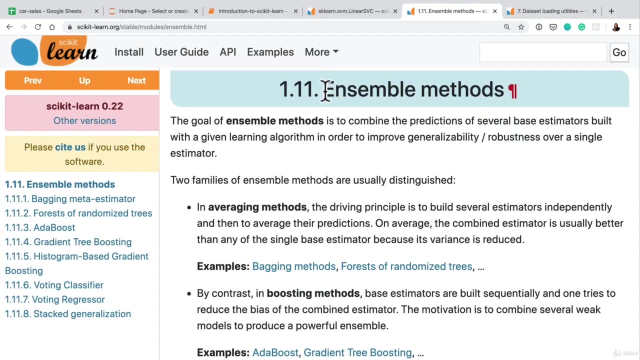 well, this is going to say K near his neighbour's classifier, but I'm going to skip this one. I'm going to go to ensemble classify, so let's click on this now. why this? Because we've seen this before. ensemble methods- forest of randomised trees. 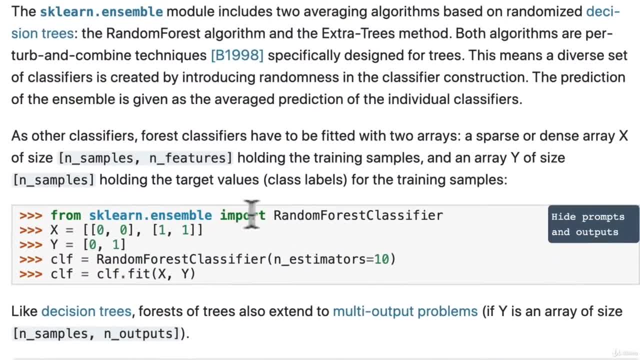 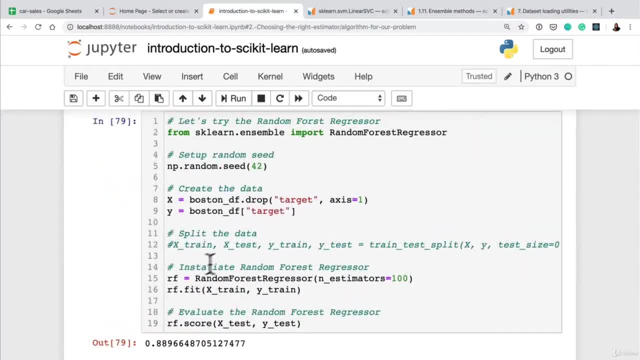 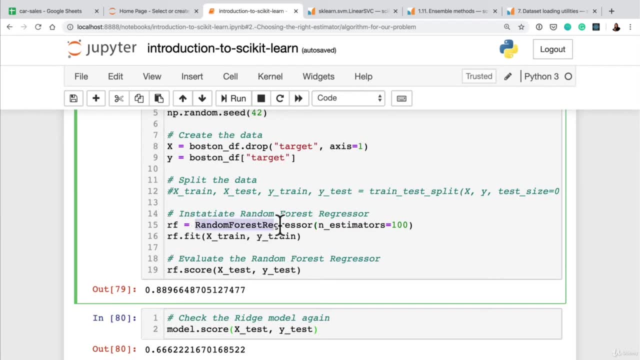 sklearn ensemble from sklearn ensemble import random forest classifier. now, if you remember, back up in our regression problem, when we switched to using a random forest regressor, we saw a bump in the score. well, because random forest regressor did so well. good news is for us: it's got a. 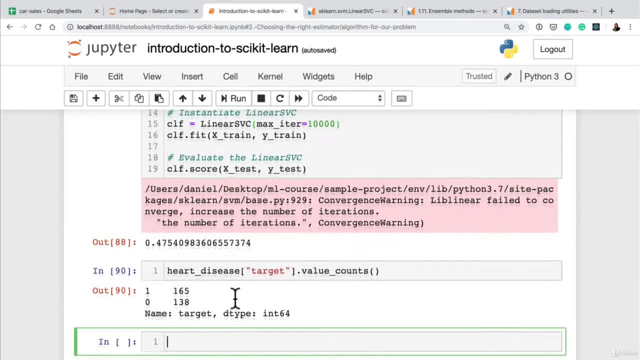 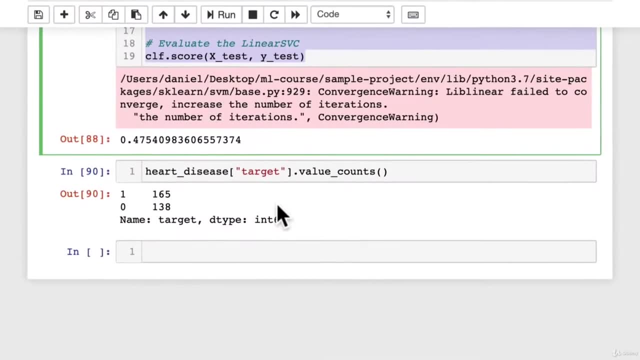 trans-partner called random forest classifier. we've actually seen this before, but what we're going to do is compare it to linear SVC. so, to save time, I'm going to copy this code and I'm going to bring it down here. so we want to change this to random. 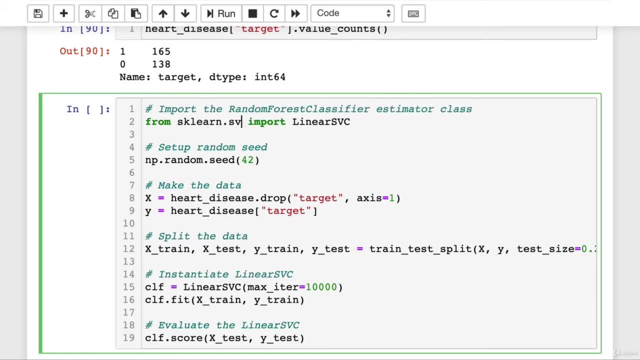 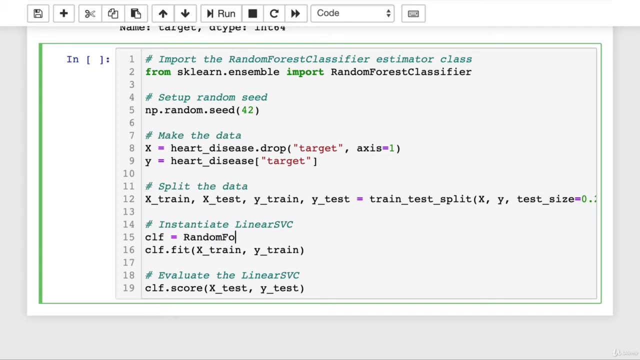 forest classifier. we actually want ensemble import. random forest classifier- wonderful. we can keep the rest the same, except for this. we need to actually sub this out: random forest classifier. and we want to go. random forest classifier- wonderful. we'll do the same here. just to tidy up our notes. keep our code. 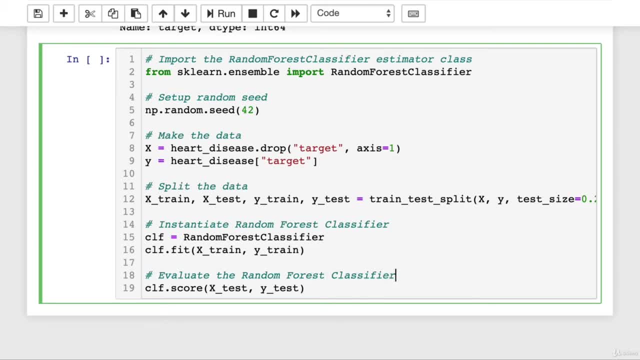 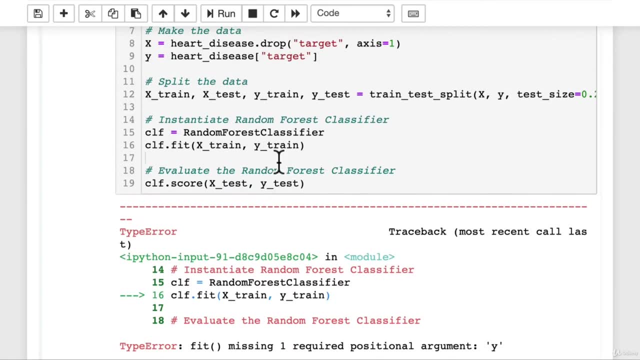 communicative. wonderful, and now what do you think will happen here? 3,, 2,, 1,. let's see error fit. missing one argument why? oh, there we go. That's what we forgot. We forgot to add the little brackets on the end. 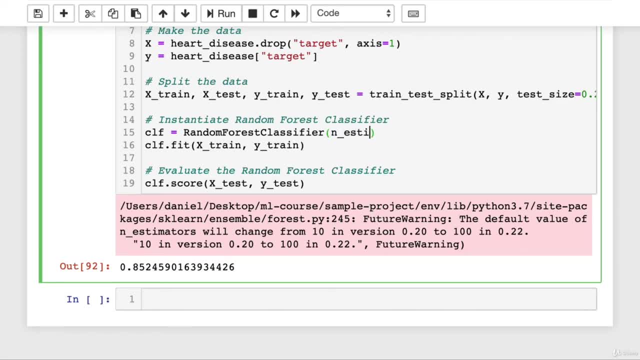 Ah, wonderful. Now to get rid of this warning, we need to change n estimators, because, see here, the default value of n estimators will change from 10 in version 0.2 to 100.. So we'll just get rid of that by changing n estimators. 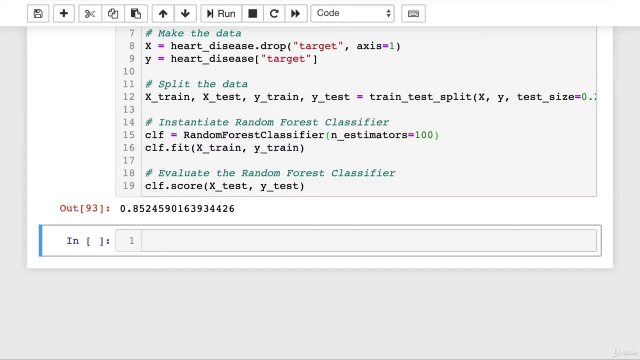 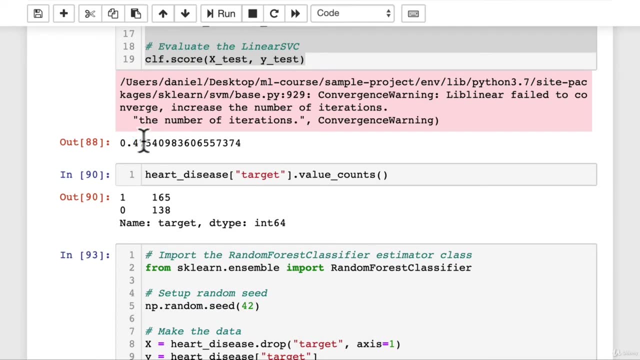 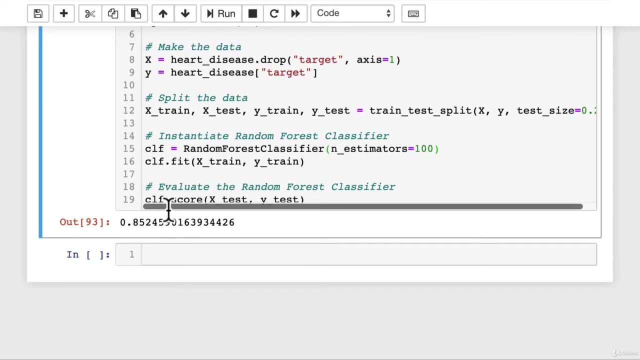 equals 100. Delicious, Wonderful. So what's happened here? We've used a different model. Now, linear SVC has scored 47% accuracy and our random forest classifier has scored 85% accuracy. So nearly double by just using another model. So you can see why I'm kind of jumping to. 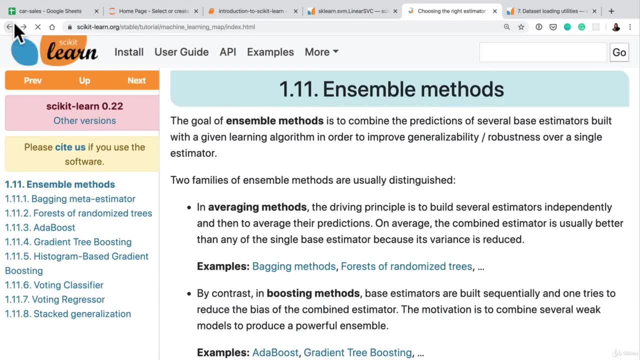 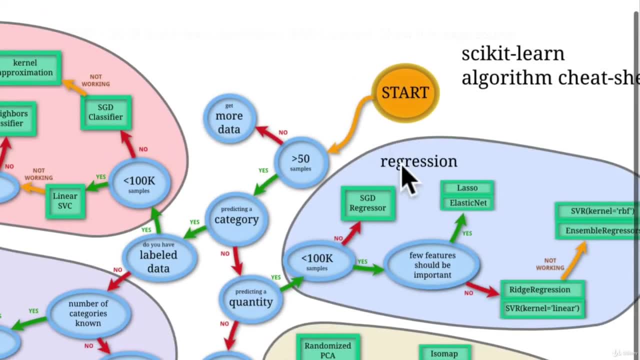 using random forest. If we go back, all I've done is I've gone start. I figured out what kind of problem we're trying to solve. You can do this as well. So for our regression problem, we were trying to figure out whether something was a number. For our classification problem, we were trying to predict a label. 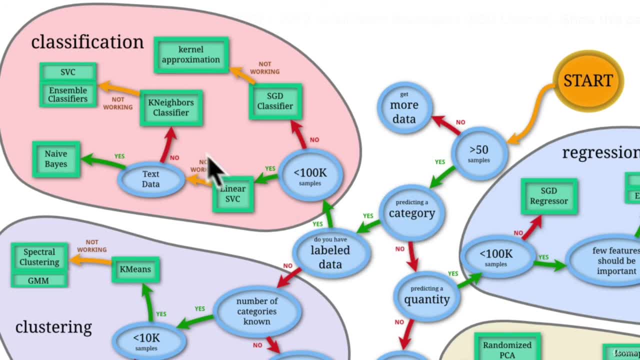 Do we have label data? Yes, Are we predicting category? Yes, And now our linear SVC model wasn't working, so we went straight to ensemble classifiers. And now you might be thinking: what about all the other models? right, So we've kind of skipped all these ones here. 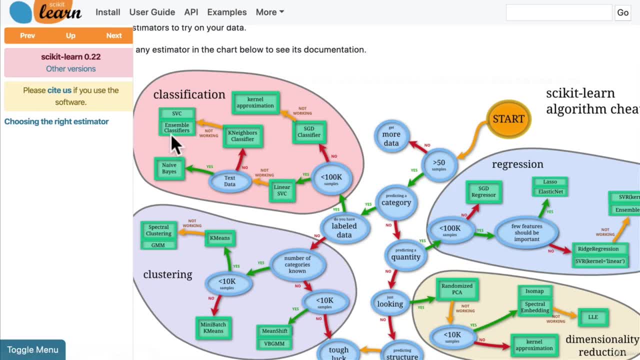 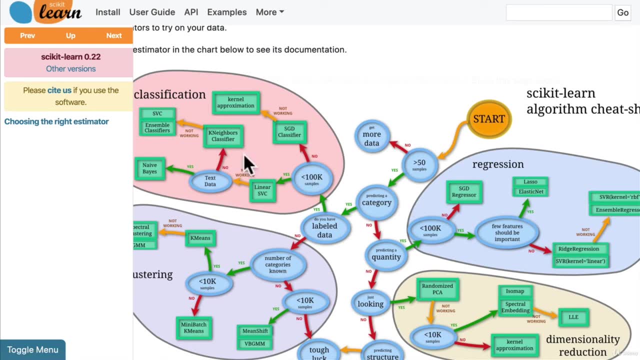 All of these And we've only really touched the surface. We've only used this one and ensemble classifiers for both, And that's a great question. Well, the first reason is namely for time. we could go through and try all of. 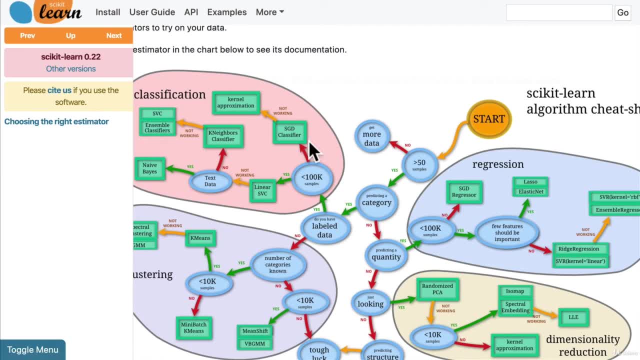 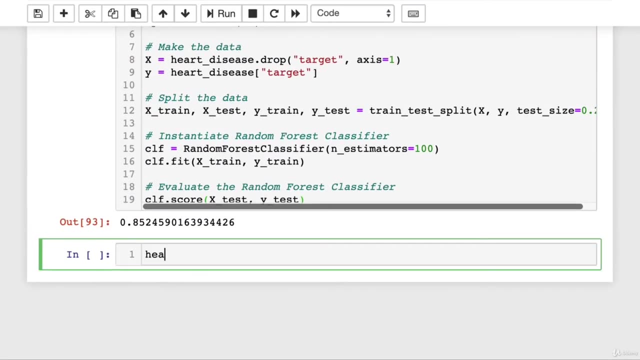 these. And the second reason is there's a little tidbit in machine learning. If you have structured data, aka tables or data frames, use ensemble methods such as random forest Why? Because it'll perform pretty well If there are patterns. this is a tidbit. 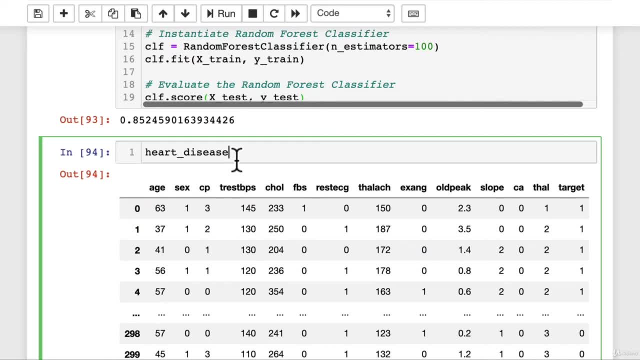 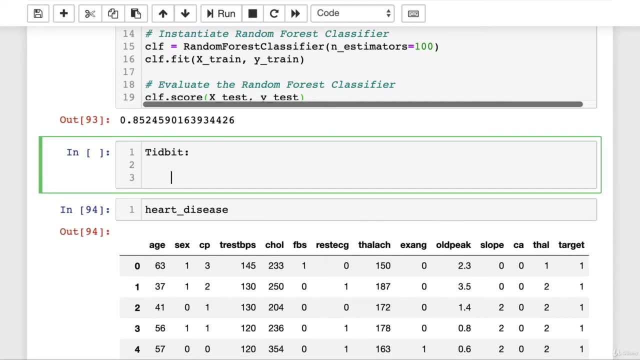 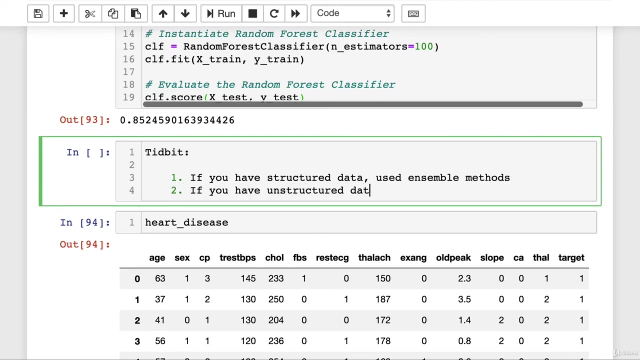 here Heart disease Might write this down, so we know I'll put this in a resources section as well. Tidbit is: 1. If you have structured data, use ensemble methods, And 2 is if you have unstructured data use. 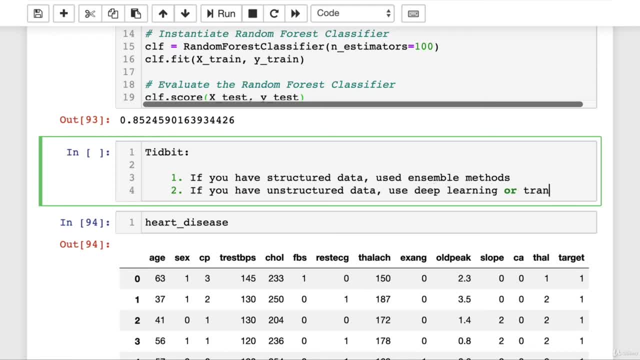 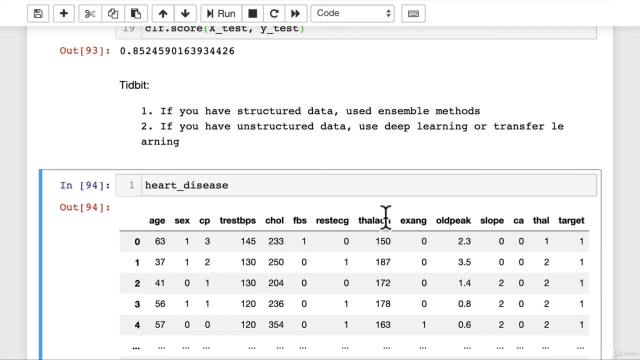 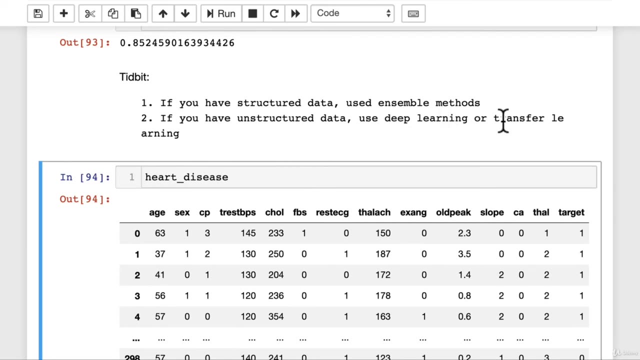 deep learning or transfer learning. Now, what's an example of structured data? Well, stuff in a table like this. And if we have unstructured data which is like images, audio or text or something like that, use deep learning.